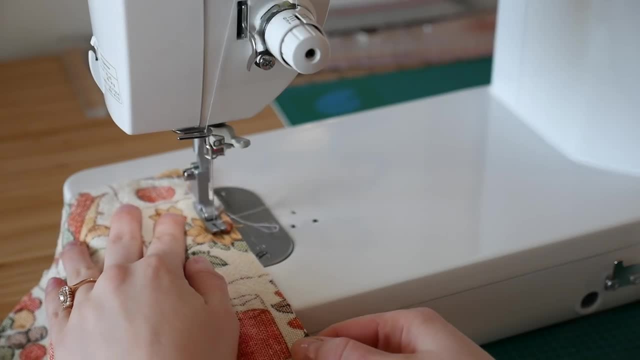 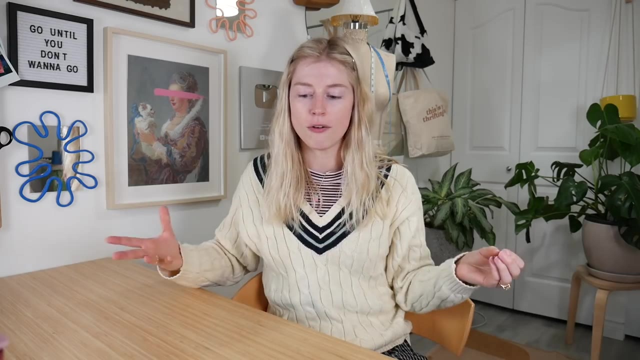 what you're learning when you're first starting to sew From there. after I learned, like my basics in my sewing class, pretty much everything else that I use is pretty much either learned online or it was a self-taught from using patterns from the fabric store and looking at the instructions. 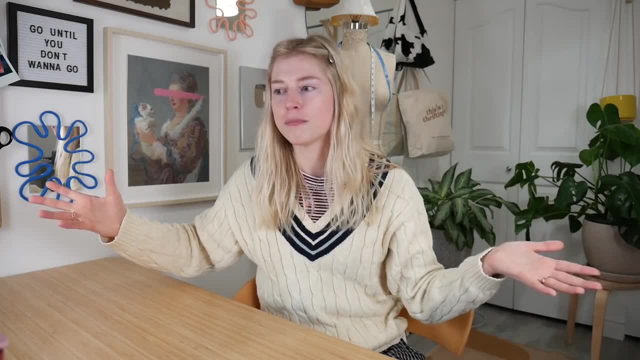 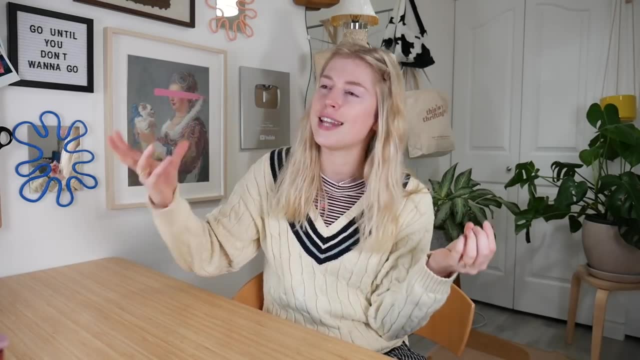 in the picture and learning techniques that way. That was pretty much how I learned. I made things and learned on the way, And that's how you really get good at learning how to make garments- and just standing it, Because when you first start you're going to see the pattern pieces and they're going. 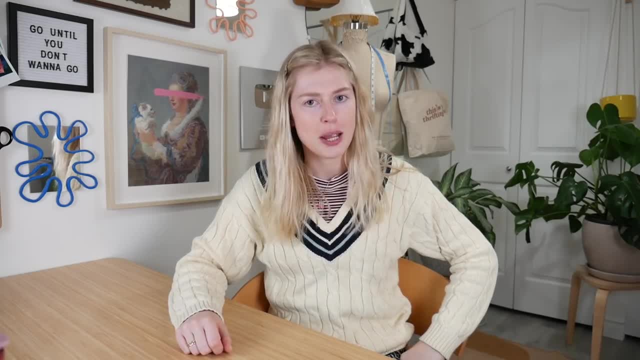 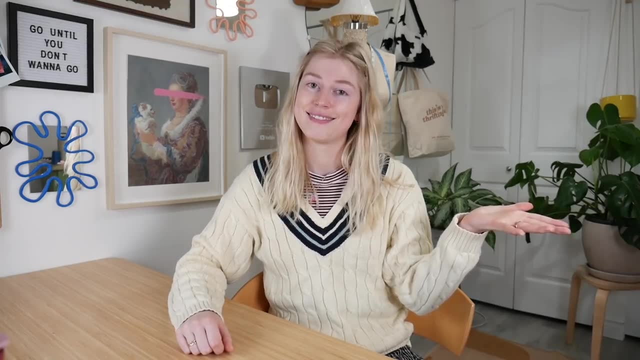 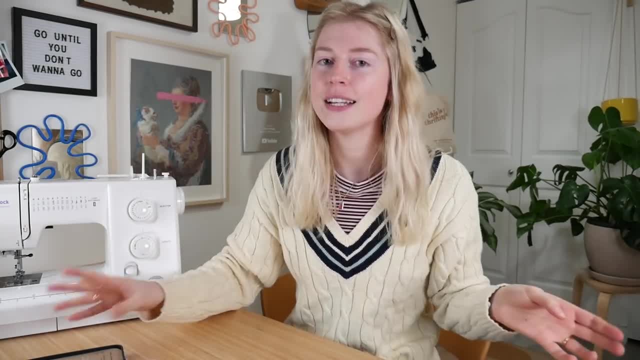 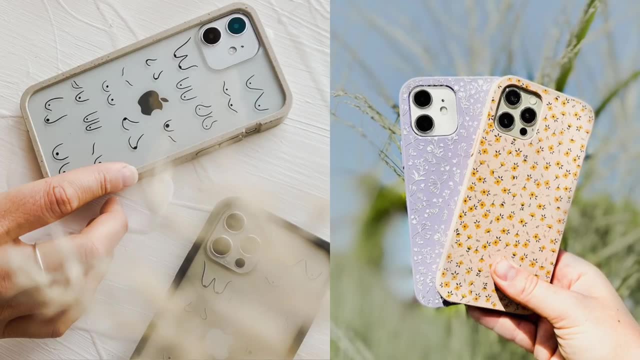 Pila- If you haven't heard of Pila. Pila is this amazing Canadian company that makes these compostable phone cases. It's honestly so incredible, It's so easy to make. It's so that these phone cases right here, even this one, and, yes, their boobs on there- can just be plopped. 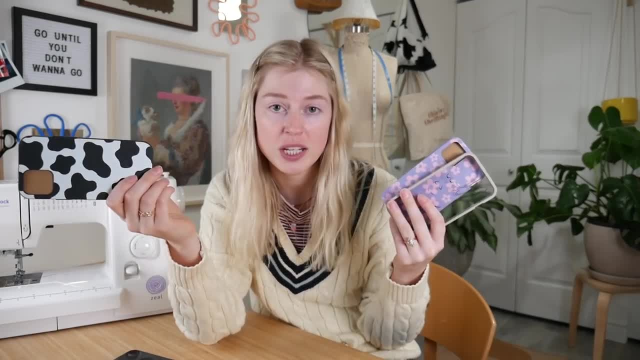 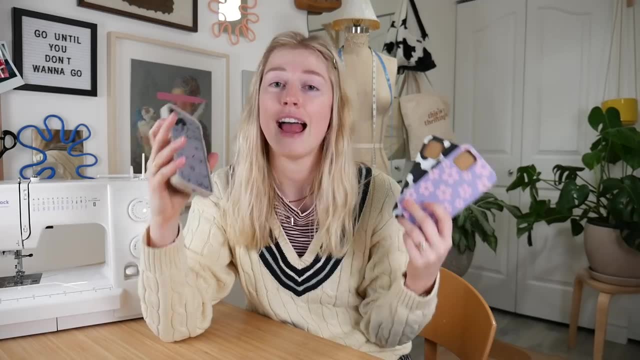 into your compost. After you get a new phone, you know you can't use them anymore. They're a hundred percent compostable. When you get your phone case from Pila, there is no plastic, There's no extra packaging involved. Everything's a hundred percent recyclable. right now, on my phone, 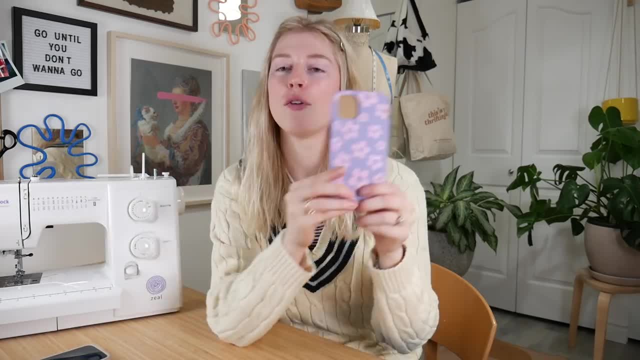 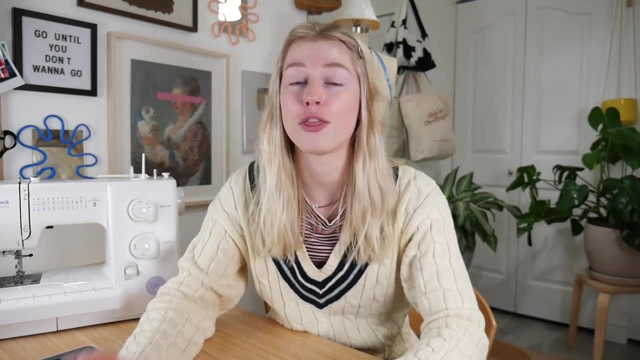 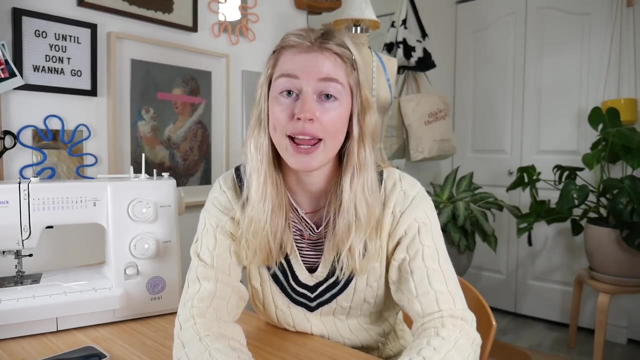 I have this amazing booby case and I also have a flower power one and a cow print one. Do you guys want to hear some fun facts? When you get your Pila case, you're actually reducing your emissions by 30%, You're reducing water waste by 34% and you're also reducing waste production by 80%. 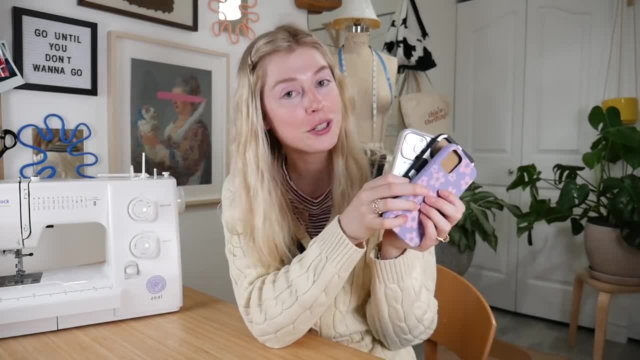 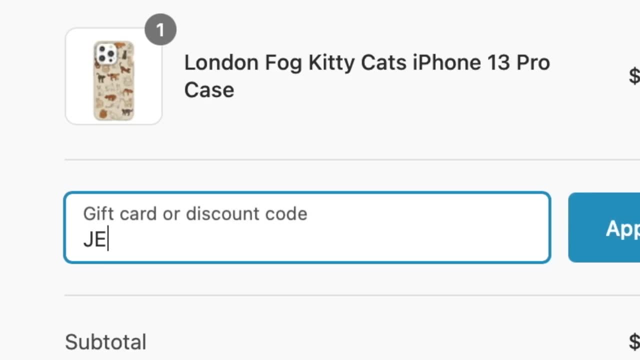 If you guys want to get your own Pila case, I have a coupon code for you guys, So the first 50 people will get 40% off and then 51 on we'll get 20.. Just use my code, JennaCheckout, And once again, 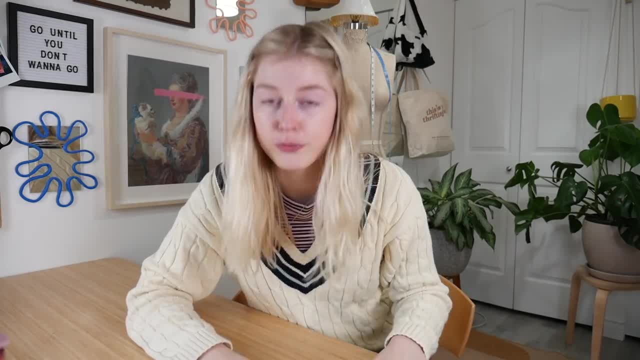 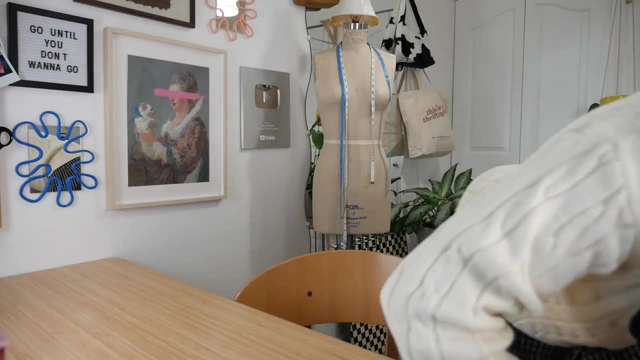 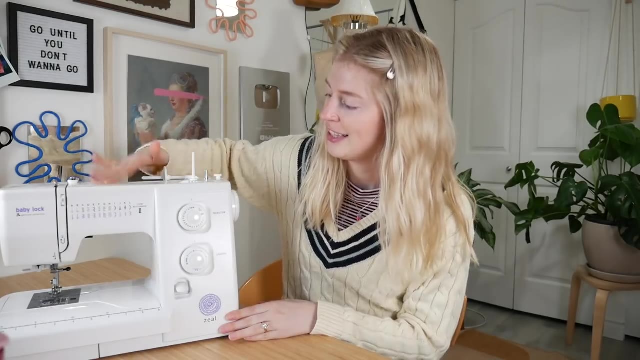 thank you so much, Pila. So for step number one, obviously we got to work on the basics. So the first thing you need- obviously you're going to need a lot of stuff- You're going to need a lot of stuff- Obviously a sewing machine, One of these bad boys, just like this one. So if you guys are 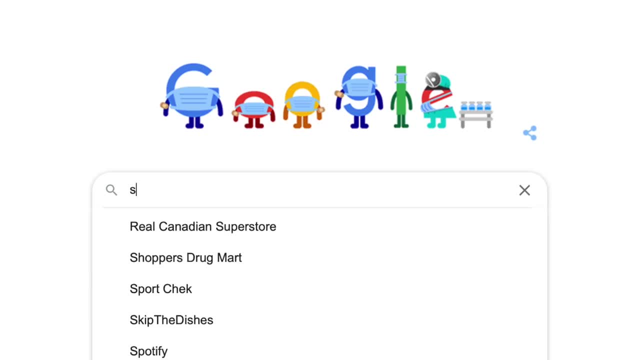 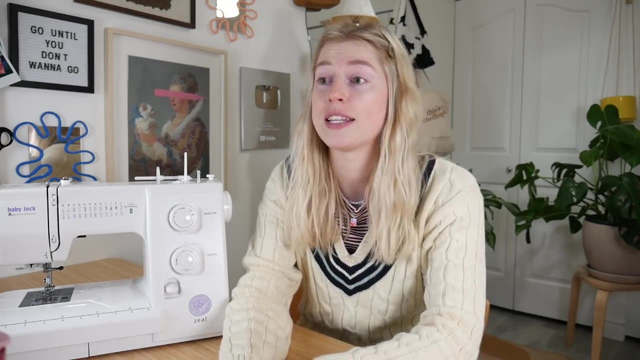 interested in sewing. you've probably all done this. You looked up on Google, you typed in sewing machine and then you just got a huge big list of results of sewing machines. And then you probably went best sewing machines And then you just got a huge list of results of the best sewing machines. 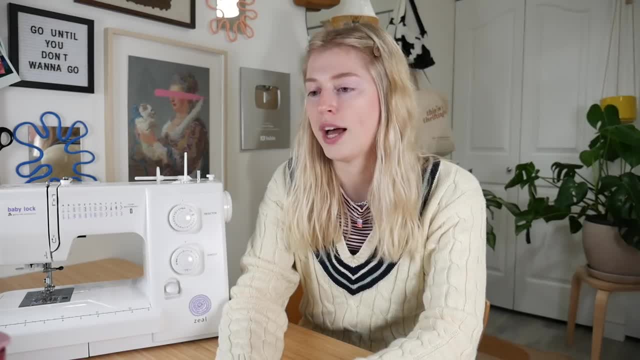 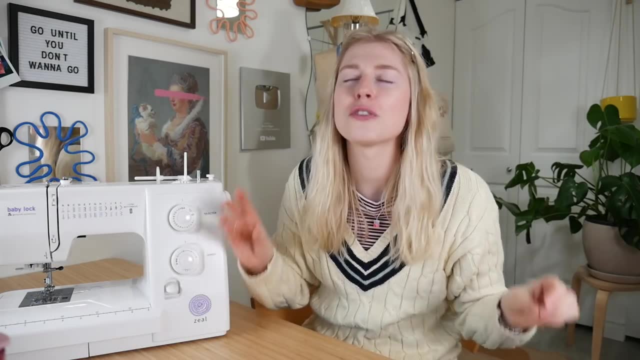 out there And, um, you couldn't get a clear answer. And that's what I've been doing for the longest time I did, And really there's no best sewing machine out there. There's a lot of good ones. Like, there's so many sewing machines out there that you can't just say this is the best. 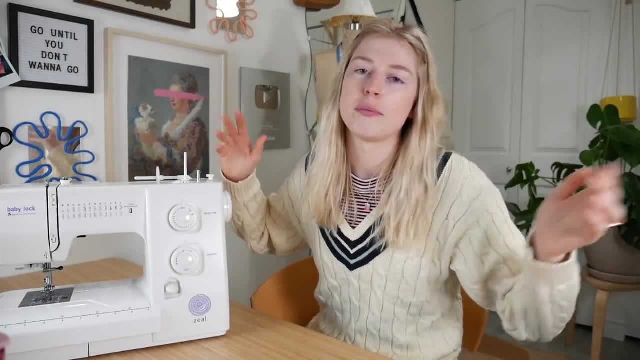 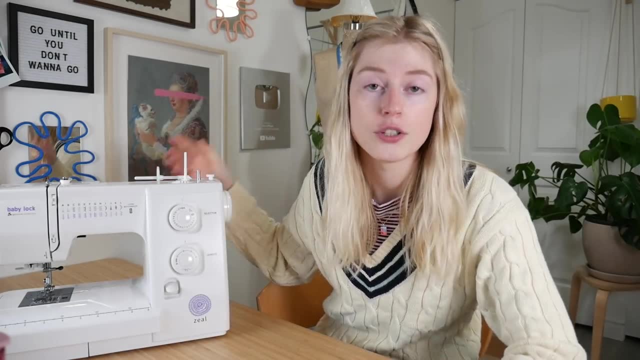 one for beginners and everyone should get it. It's just like impossible, but mainly for beginners. you just want a basic sewing machine. You do not. Okay, The one thing you do not want is you do not want one of those little baby sewing machines that are probably like 20, $30. And they're just like. 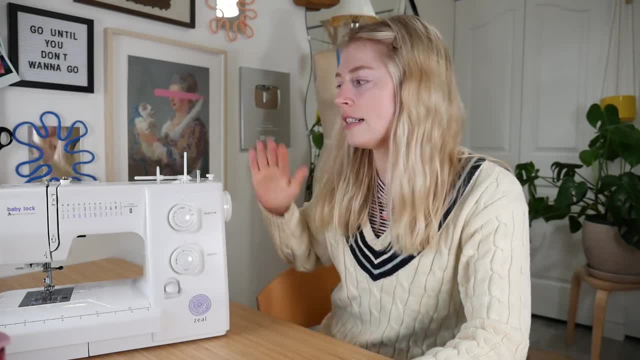 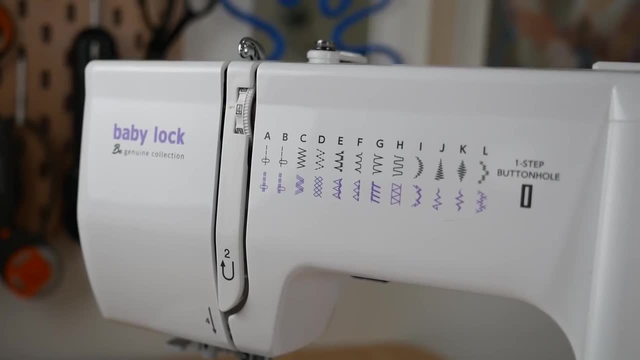 this big. Don't get those. Don't get those Like: at least get a decent one. So when you're looking at sewing machines, you want a sewing machine that pretty much has a decent amount of stitches. You don't want one that just has like. 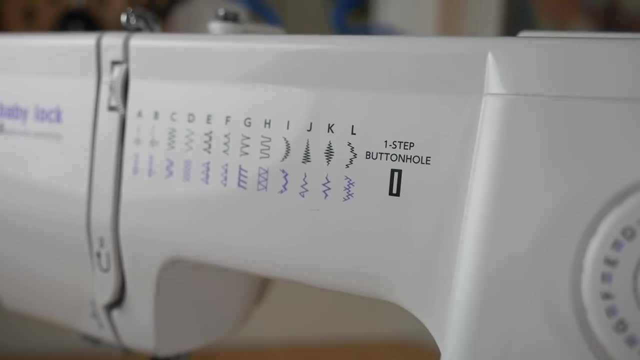 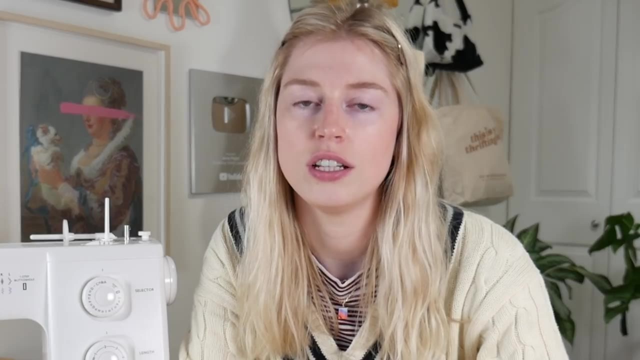 two stitches Like you want, one that at least has a straight stitch, a zigzag and a buttonhole. Those are like the three important ones. But if that didn't really help and you're still like Jenna, I just need an answer. What sewing machine to buy? I did a little survey on my Instagram. 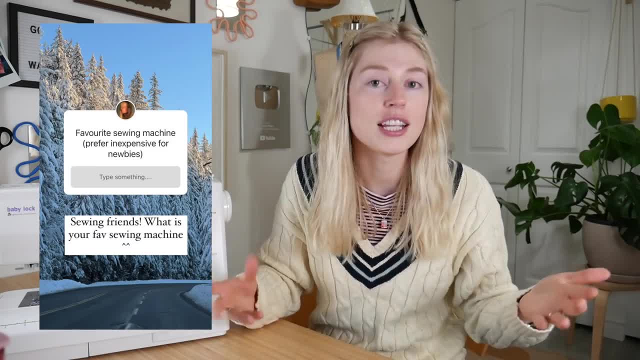 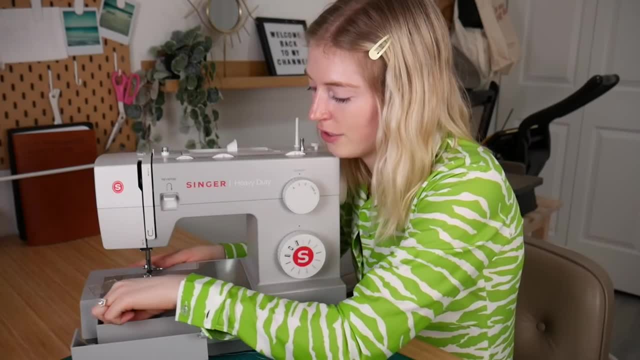 asking everyone what sewing machines they had, or their favorite, And the number one that came up was the heavy duty one. I personally had this sewing machine before I upgraded and it was amazing to start off with, Like it was a good, decent sewing machine that did everything you. 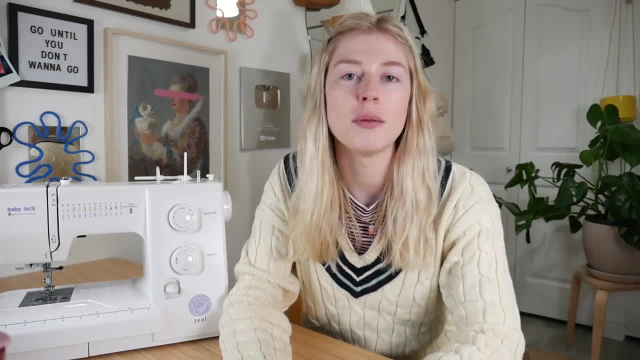 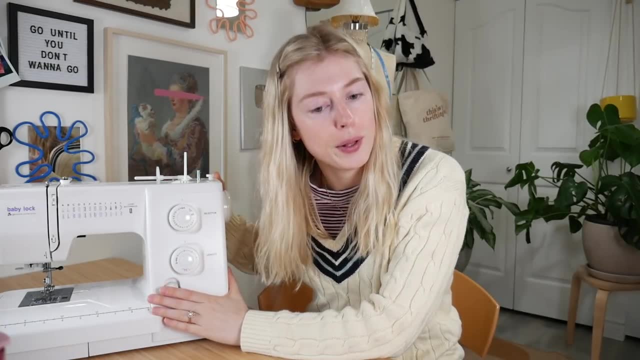 need for the basics, Like you don't need anything else, And that one is pretty much available everywhere, everywhere, So that's a good one. Now you're probably going to wonder, Jenna, why don't you have that sewing machine? Well, I mainly use a semi-industrial one, So like a real heavy duty. 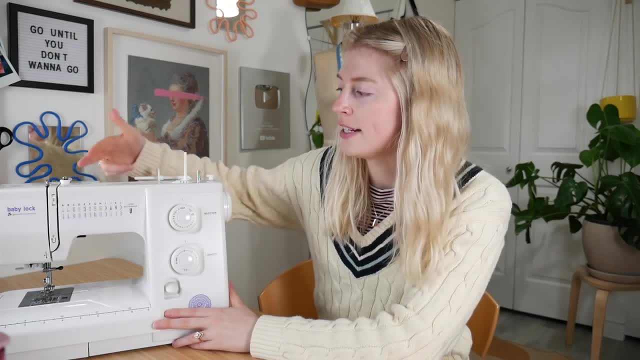 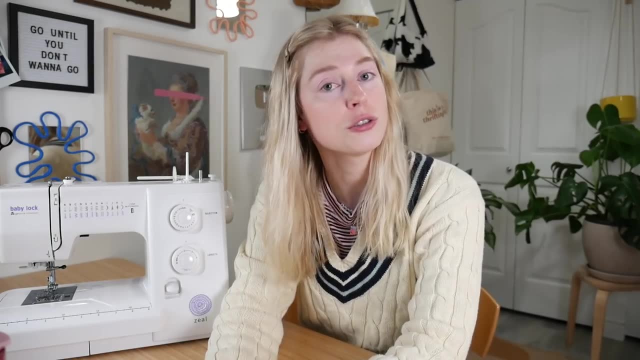 one that can sew through like anything. And then this is like my backup, one that I can do like zigzag buttonhole. I'll link it down below. but I know there's going to be some of you out there that are like I can't afford a $300 or $400 sewing machine or $200.. And you don't want to because you're like: 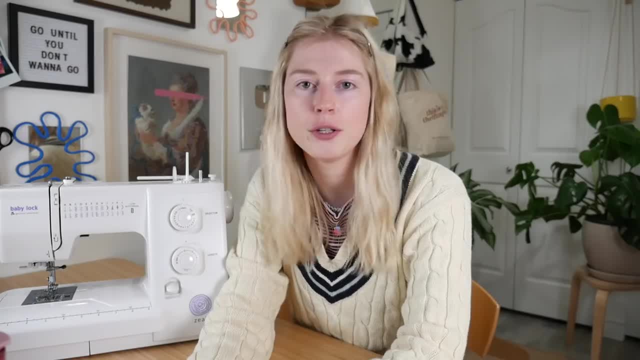 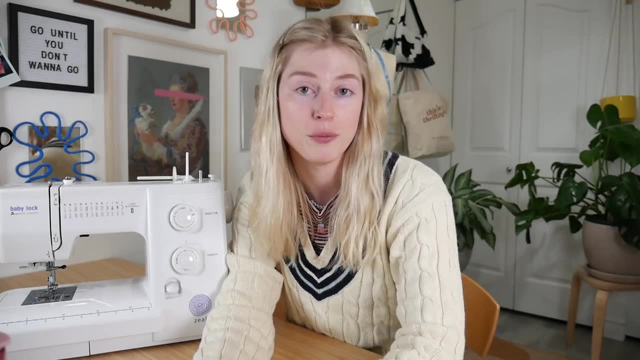 I don't even know if I'm going to like sewing And I don't recommend buying a brand new sewing machine off the bat. I didn't. I used my mom's old sewing machine probably for like three to four years before I even thought about buying one, And it was great. So you guys can definitely find a. 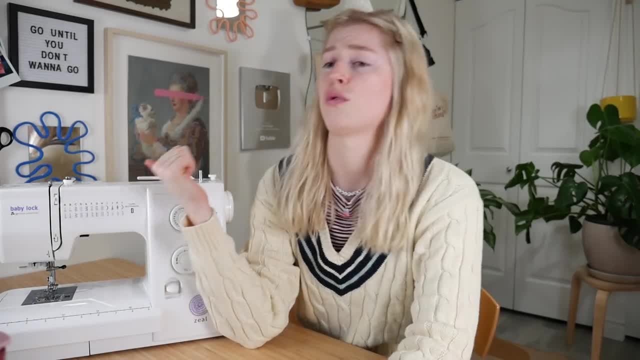 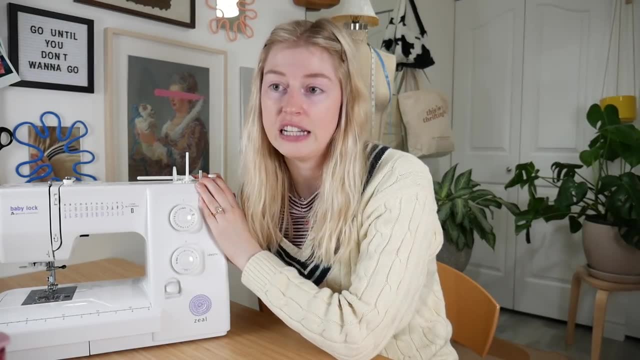 secondhand sewing machine, either on Facebook marketplace or at your local thrift store, or even borrow, like your grandma's- She still has one Anyone. but other than sewing machines, you definitely need other things, Unfortunately, and you're like you need a lot of supplies, Like you need pins, you need thread, you need. 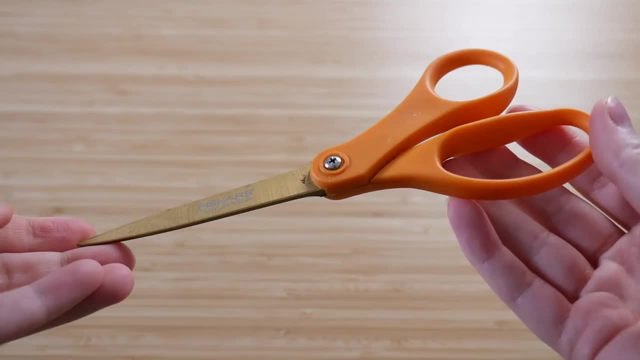 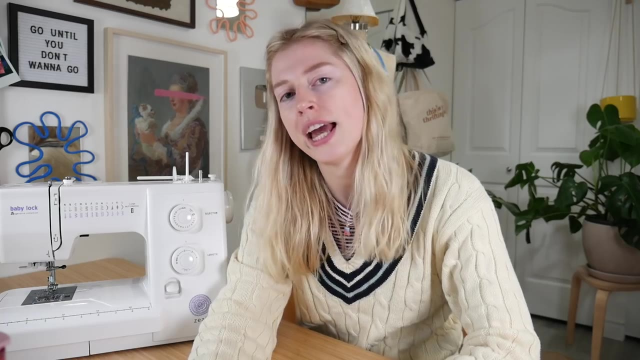 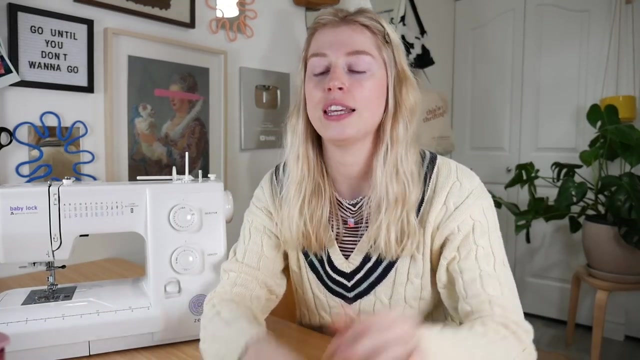 hand sewing needles. You need scissors- one for paper and one for fabric. You need an ironing board. You need an iron tape measure and a safety pin, but you might already have one of those. There are more notions sewing things that you probably need if you're going to keep going and 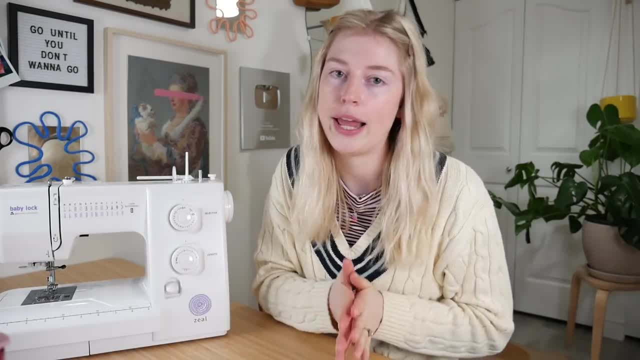 sewing, but those are like the bare minimum basic ones that you're going to need. So, if you're going to keep going and sewing- but those are like the bare minimum basic ones that you're going to need- want to have. So now we're going to need something to sew with, And what I recommend for beginners. 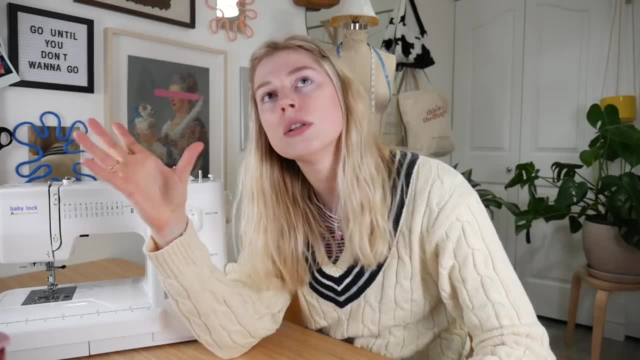 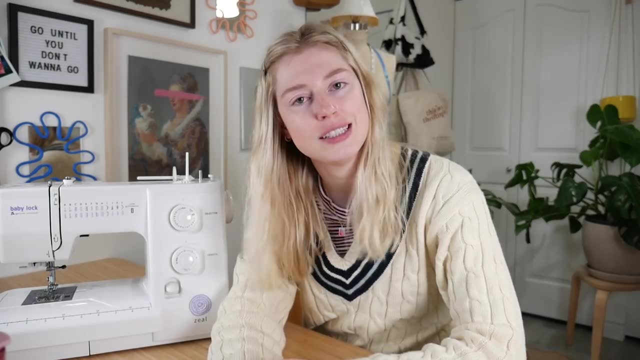 is a hundred percent cotton fabric. This fabric, I know it's not like the most luxurious fabric, You're not gonna make a wedding dress with it, but it's practical for beginners. It's really easy to work with, It's easy to iron, It's nice and smooth. It won't like move a lot, It's just. 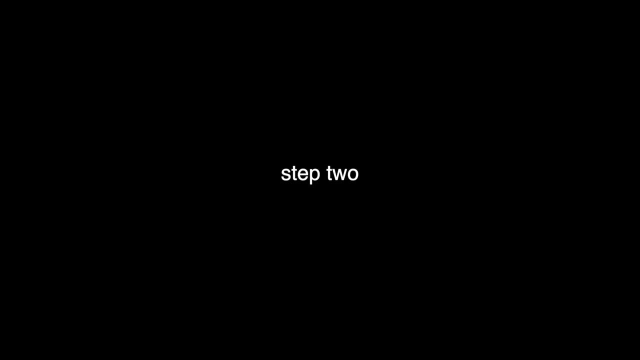 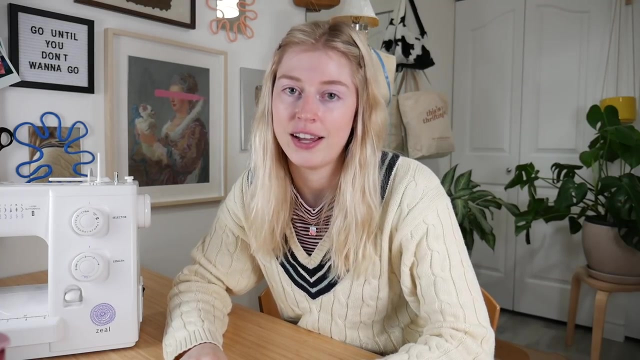 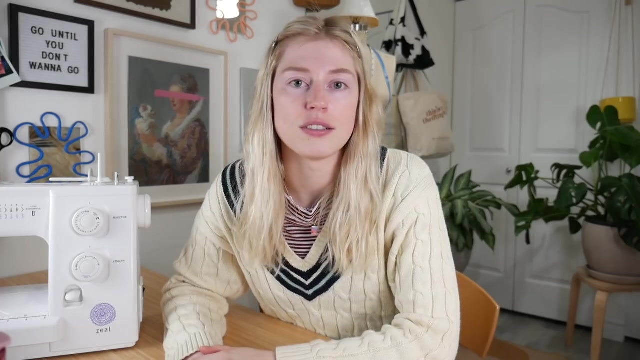 your best friend when it comes to beginning. So step number two: this is where it gets interesting, kind of fun, kind of terrifying, because now we actually need to learn how to use this bad boy over here, And I know it's. this is the intimidating part. We're getting down to business. 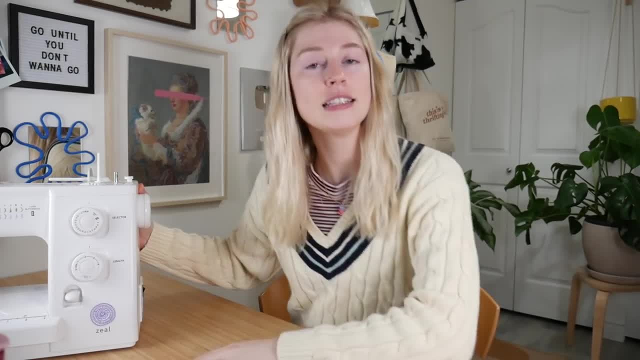 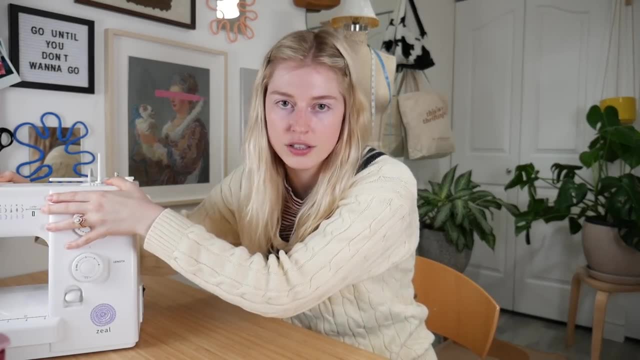 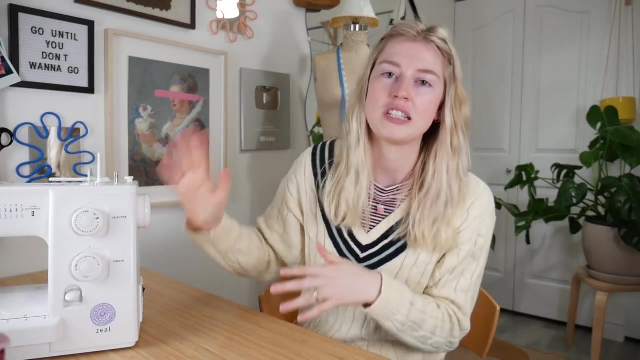 So learning the machine, understanding machine. it can take a little bit of time, but I found the best resources of how you guys can learn how this works, how to thread it, understand it. just understand her Cause she's a little confusing if you've never even seen one or seen one. 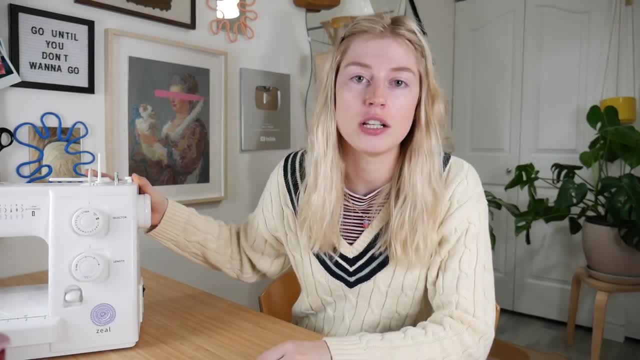 being used. Pretty cool, And then you can learn how to use this. So that's pretty much. 95% of these machines are like thread, the same line and set up pretty similar, So you don't need to find a specific torp to tort. 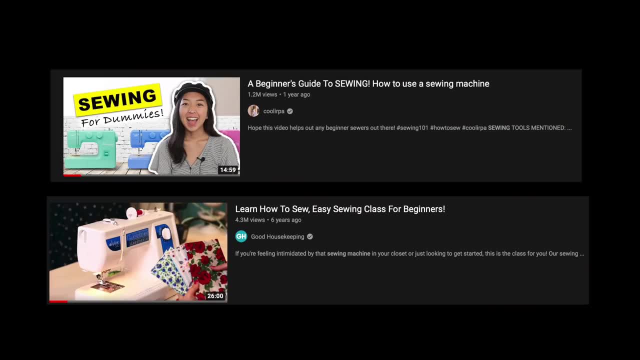 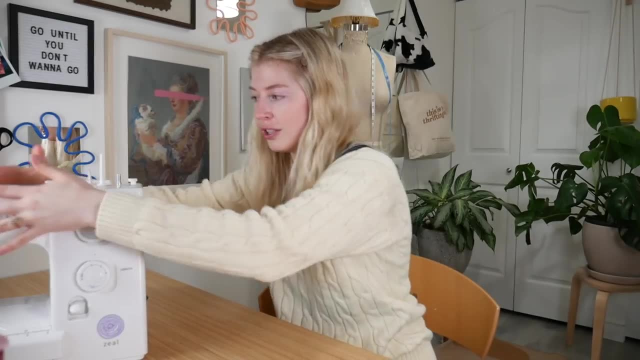 tutorial for your machine. These ones I just showed you will work, And if you have a fancy one or like a vintage one, then you fall in that like 5% category. Once you learn the machine, you understand your machine. The two things I would practice on just a scrap piece of fabric: 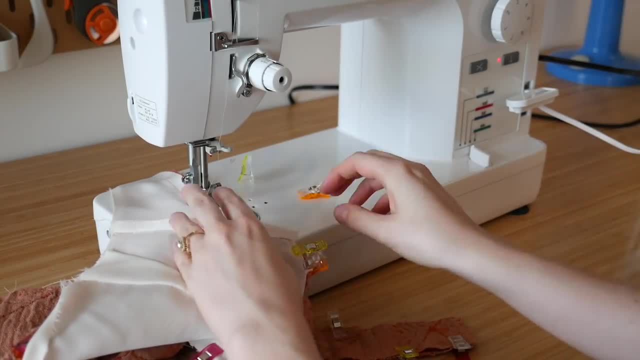 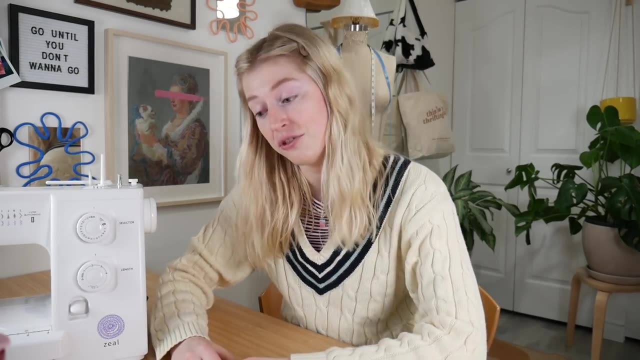 is just doing straight lines, Just keep going back and forth, sew it up and just practice And also practice zigzag stitch, doing a straight zigzag stitch. After that, and you're like I am so good at sewing a straight stitch on my fabric, Then you can start learning how to sew. 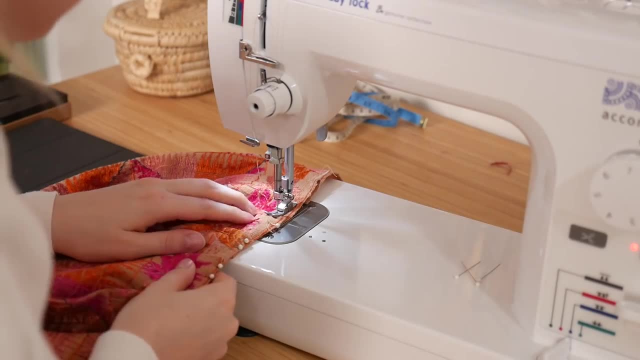 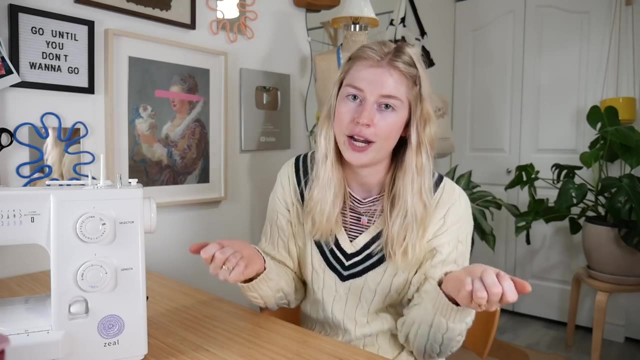 two pieces of fabric together, make sure they're lined up, have a nice seam. That's the next step. Then, after that, you can learn how to do a zigzag on the edge of the seam So it doesn't fray You. 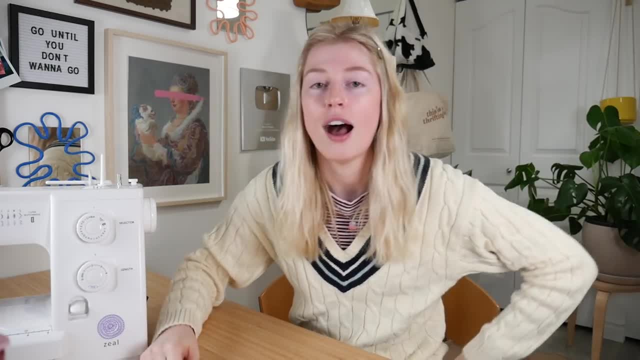 can also use pinking shears, which was like a bonus item. I don't have pinking shears because if you don't, you know, finish the edge, you're not going to be able to do it, You're going to. 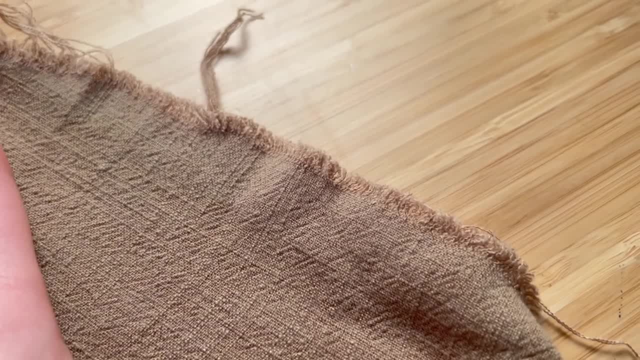 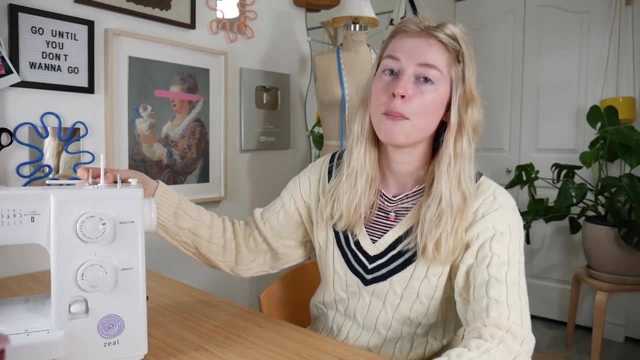 not be able to do it. So it's really important to have a nice edge of your fabric, especially if you're using 100% cotton. It's going to fray and it's going to go everywhere. It's not going to be that nice. Now for step number three. So now that you're amazing at straight stitching- 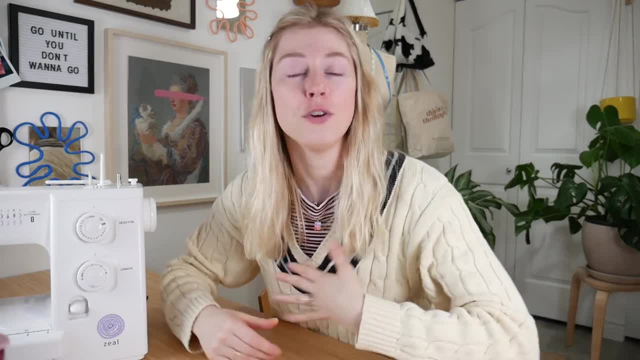 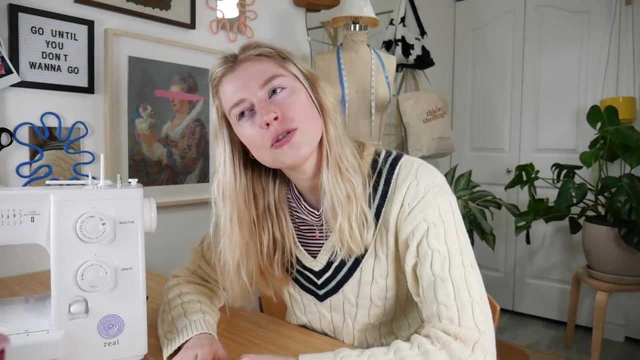 you can work on your first project. So for my first project I did boxer shorts, like I mentioned. not great, not terrible. I wouldn't start with boxer shorts, unless you're like an overachiever and you kind of understand it already. then that's a. 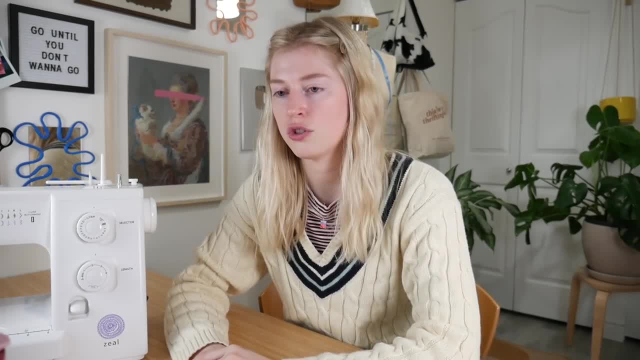 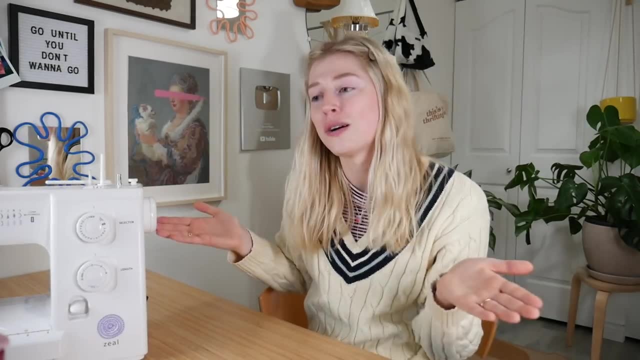 great first project, but for people that are not overachievers and just want to, you know, have a decent smooth sailing when it comes to sewing, i always recommend a tote bag for your first one. you don't have to do any curves, you're just sewing straight lines and you get a tote bag out of the 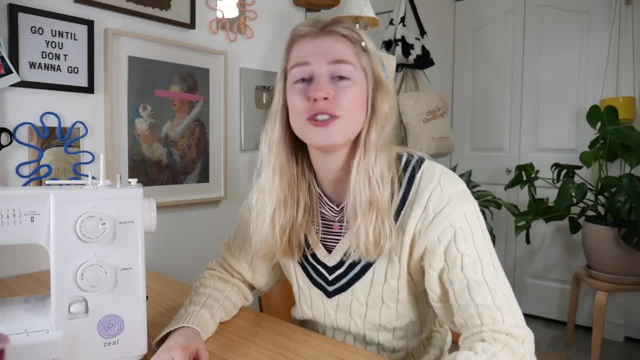 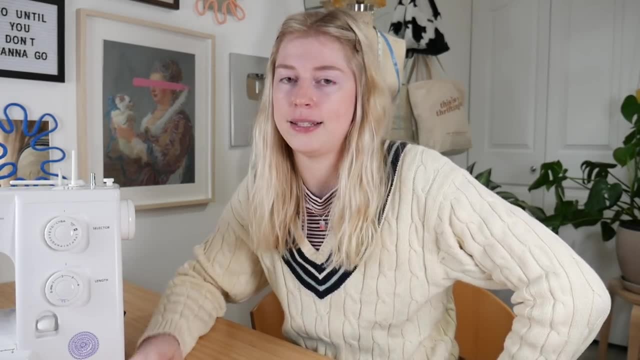 project. but if you don't really want tote bags or you don't want to make it and you're like jenna, i'm an overachiever and i don't think a tote bag is, you know, a great first project for me, because i'm amazing, then you could make a pillowcase. that's a good first project, pretty much just a. 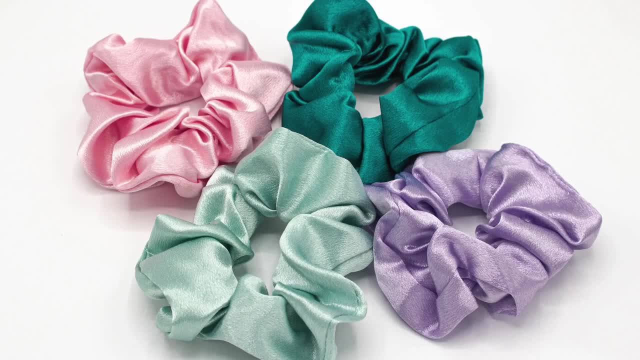 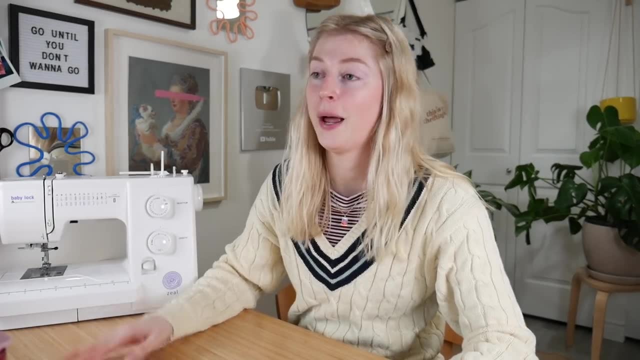 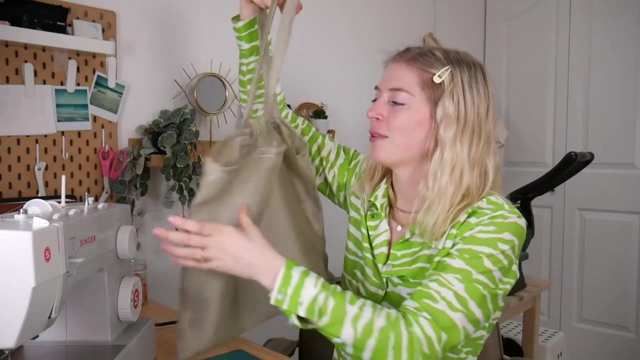 rectangle, you're sewing a scrunchie. that's also another easy one- pj shorts, like i mentioned, or sweatshorts, which are pretty much the same thing. okay, so for step number four. this is the part where you can actually start making your own clothes, after you made your first basic tote bag. 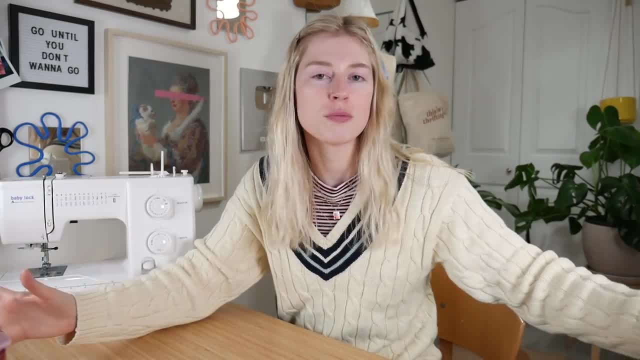 or boxer shorts or scrunchie or whatever. your first project is: now that you got one project under your belt, i feel like you can move on to actually making your own clothes. but you're not going to just make your own clothes. you're going to make your own clothes. you're going to make your 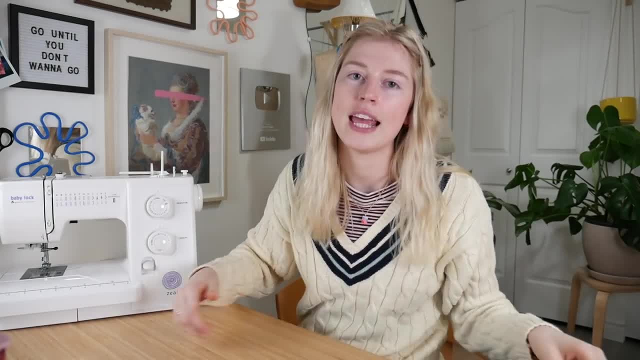 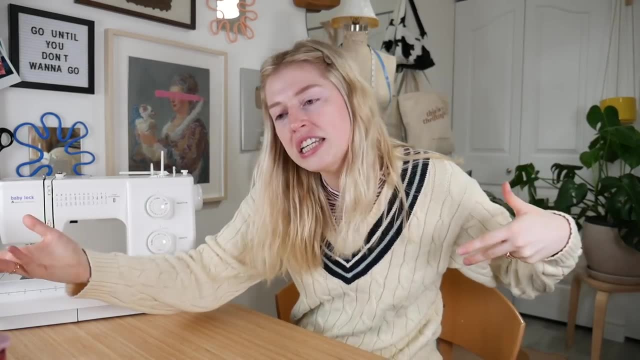 your own clothes. you're going to make your own clothes. you're going to make your own clothes just out of thin air and just draw a pattern, you know, wing it and then it's going to fit perfectly. i don't think so. you're definitely going to want to find a beginner, easy peasy, friendly beginner that didn't. 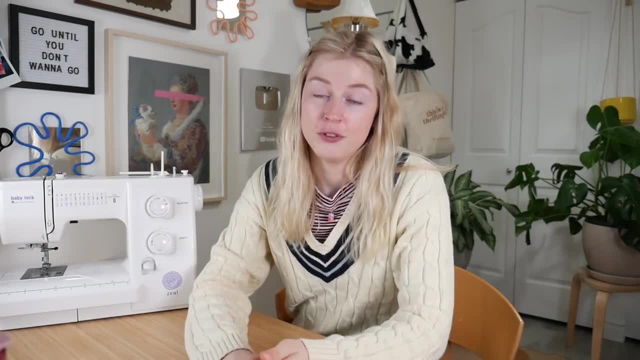 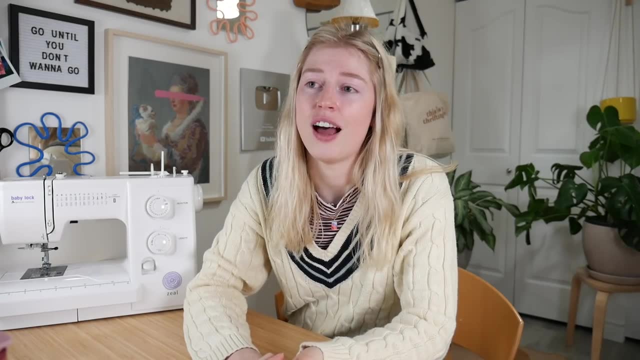 really make sense. you just want to find a beginner pattern. there's a few places you can find this pattern. one is pretty much like the old-fashioned way now, which is sad to think about because this is how i learned was like going to the fabric store and going in those big bins and looking. 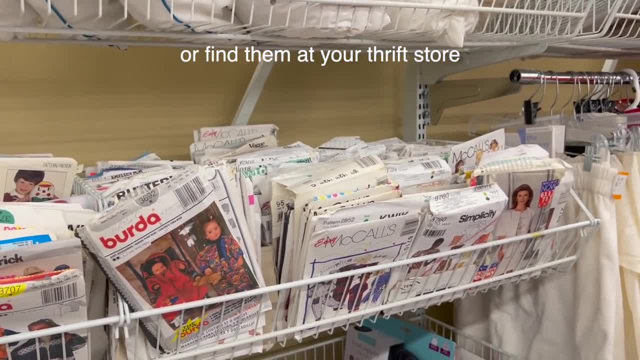 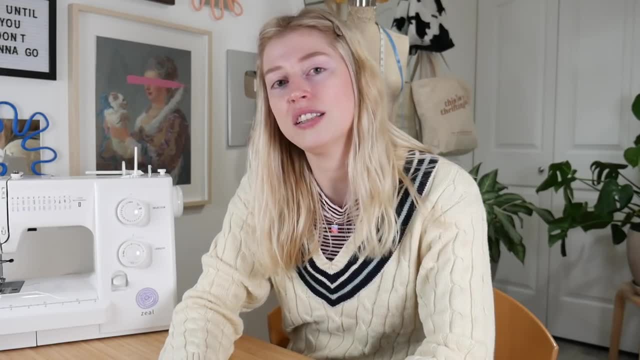 The catalog books and then finding the pattern you want. and then you go, shuffle through the bins, you know file cabinets- find the pattern And then that's how you get your pattern. But now I don't think anyone really does that, or at least personally I don't do that. 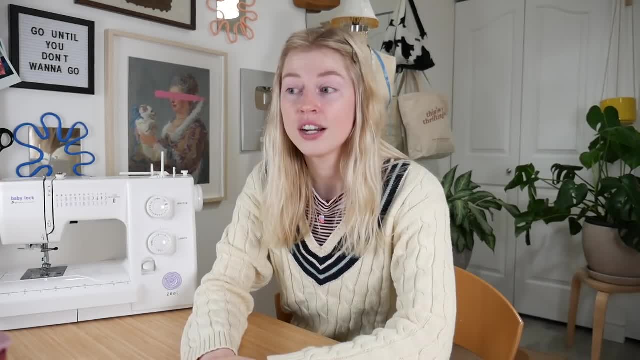 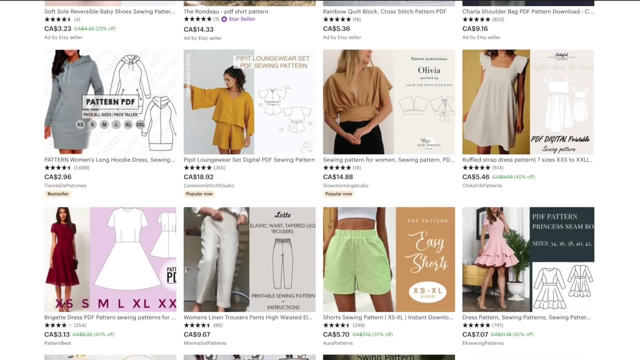 I find all the patterns I like and want to make online and a lot of them I find on etsy. That is a great resource, just because there's so many designers out there that have just amazing patterns. You can search and there's just like a huge variety of different styles on there- other places. 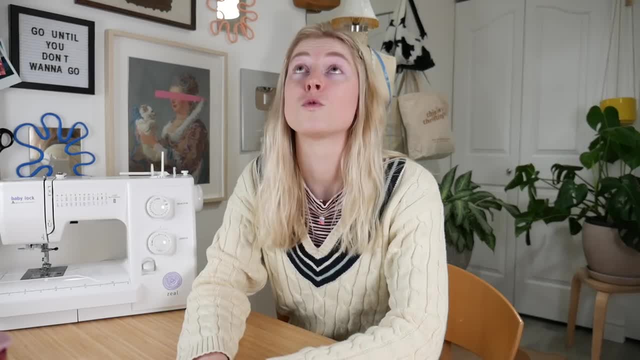 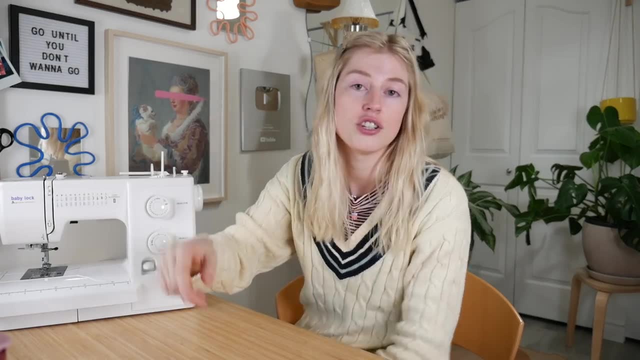 If you want free patterns, mood fabrics is a great one. They have so many free patterns on there, from beginner all the way up to intermediate, So you can just like go through the page by page, by page Page and find tons of patterns on there. I've also made a video with my favorite free patterns. 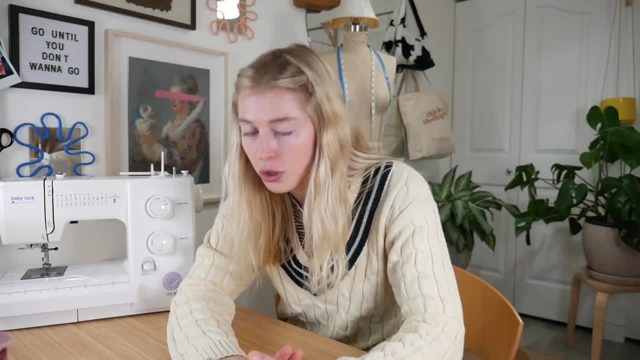 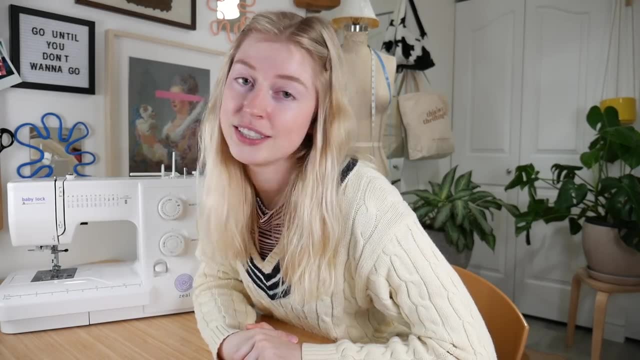 I'll link it down below so you guys can check those ones out. and then I also Curated some patterns here which I thought would be great for beginners. Well, that's it. So I hope you guys enjoyed today's video and got some inspiration, some motivation to get started on.